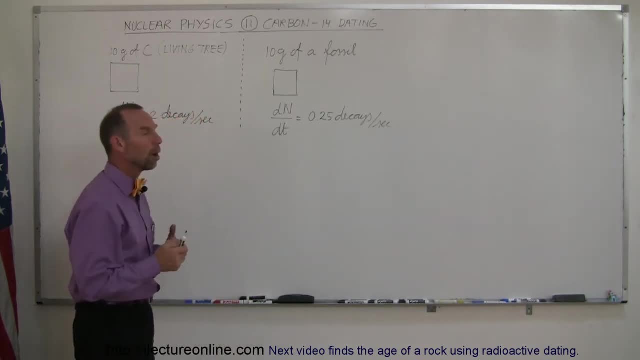 rate is only 0.25 decays per second. So how old is the fossil? Well, first of all, we realize that the amount of radioactive material that's left as a function of time is equal to the original, that you started with, times e, to the minus lambda, times t, Now, since the decay rate. 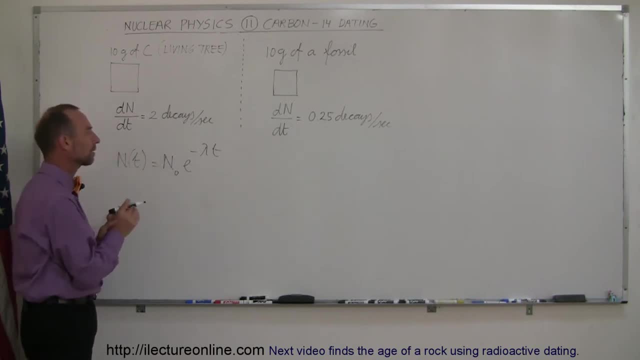 is proportional to the number of radioactive atoms in the fossil. we can say that the decay rate is equal to the amount of radioactive atoms in the fossil. So we can say that the decay rate is equal to the amount of radioactive atoms in the fossil. So we can say that the decay rate is equal to the amount of radioactive. 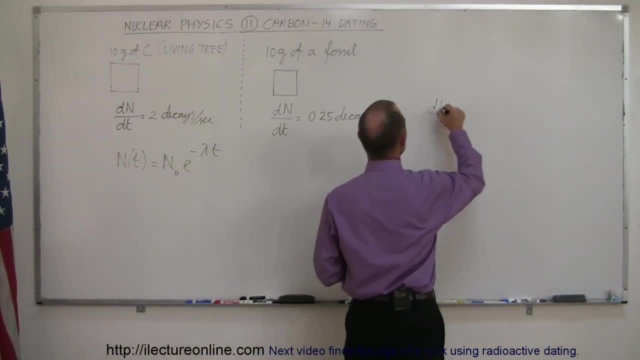 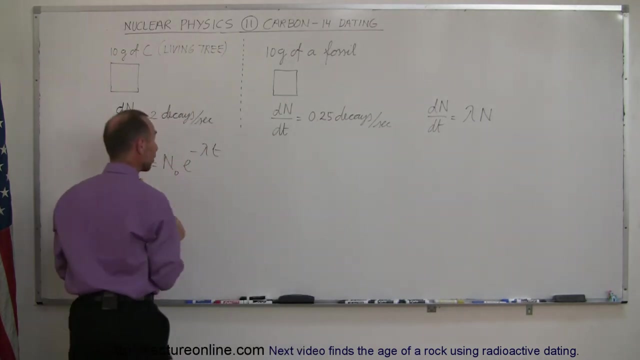 You know, just make a e to the minus lambda times n, to the times we define the deno line nuclei in the sample. remember that the dn dt is equal to lambda times n. so we can then say we can replace the n and the n sub-naught by the dn dt and the n? dt sub-naught, because they're 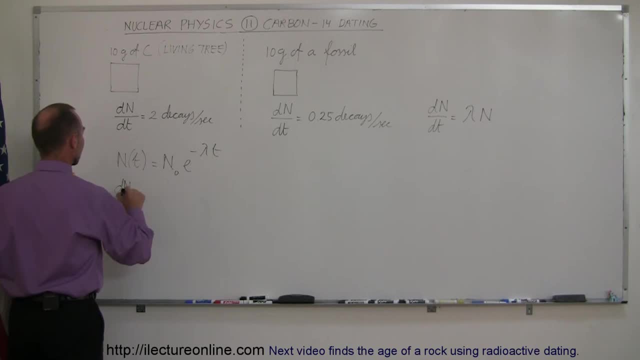 proportional anyway. so we can write that the rate – the dn dt of the sample is equal to the dn dt of the original test sample sample, and let's call this dn dt, like that, times e to the minus lambda times t. Now, of course, 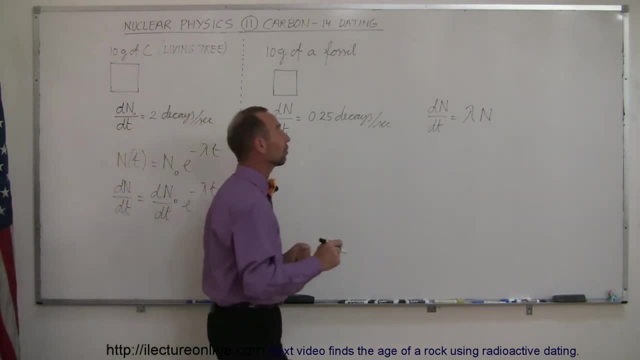 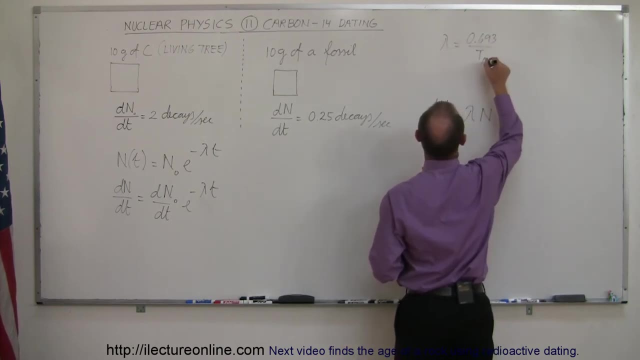 we still have to find lambda. I know we've done it before, but just for practice let's do it again. The decay constant is equal to 0.693 divided by the half-life. So that's equal to 0.693 divided. 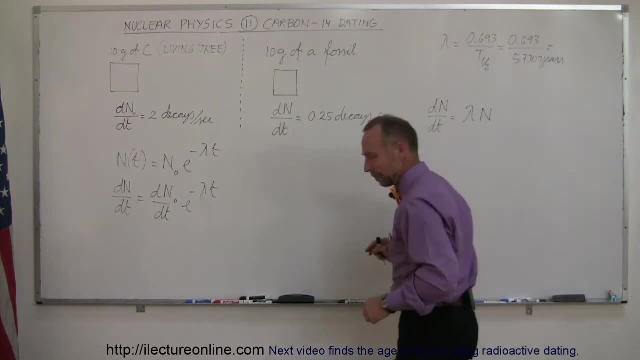 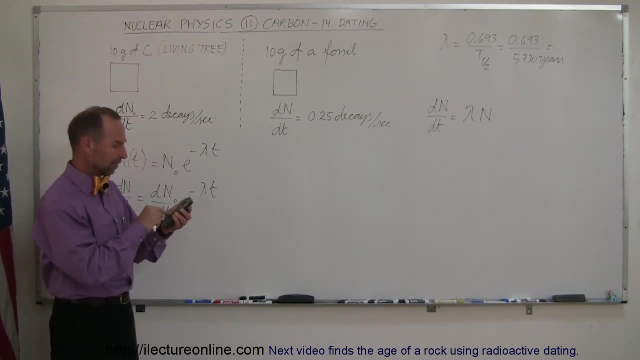 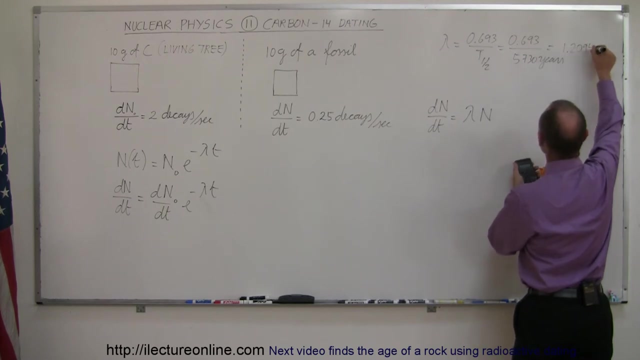 by 5,730 years. So if we grab our calculator we can figure out what that is. So 0.693 divided by 5,730 equals so that would be 1.2094 times 10 to the minus 4 per year. 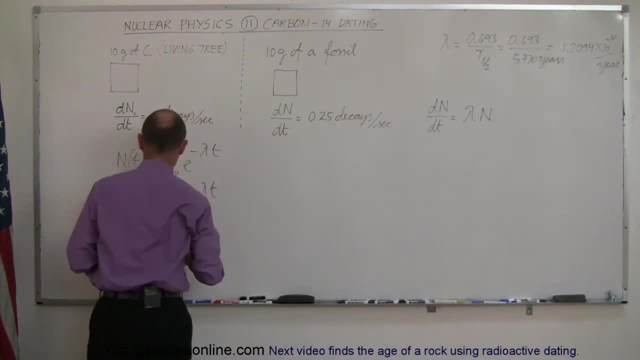 So that's the decay constant for carbon-14.. Plug in the numbers here. let's see what we get. here We get 1.2094 times 10 to the minus 4 per year. So that's the decay constant for carbon-14.. 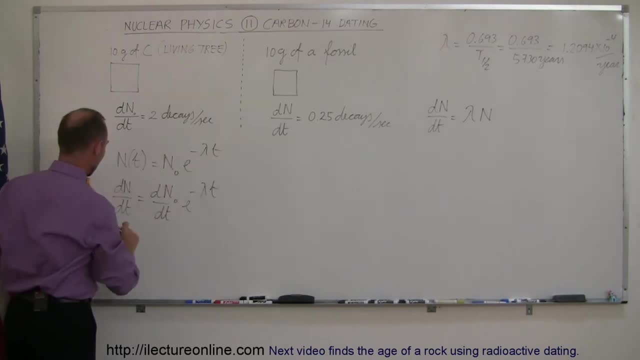 we get. that's the decay rate that we currently have in our sample. so 0.25 equals the decay rate that we have from the first sample, which is 2, times e to the minus. the decay constant is 1.2094 times 10 to the minus 4 per year times t. And what we have to do here now is: 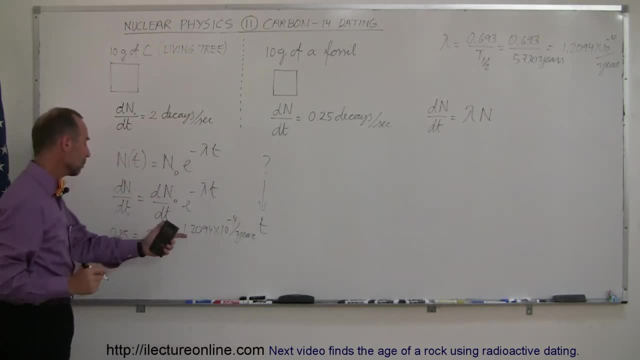 figure out what the time elapsed is, what t will make this equation come out like that. Alright, well, first, what we're going to do is divide both sides by 2, and 0.25 divided by 2 is the same as 1.8, because 0.25 goes into 1 four times, so it goes into 2- eight. 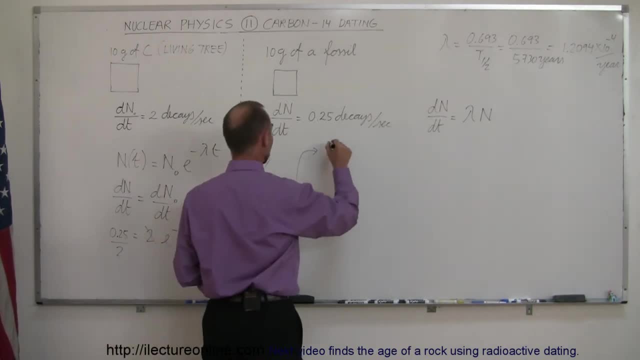 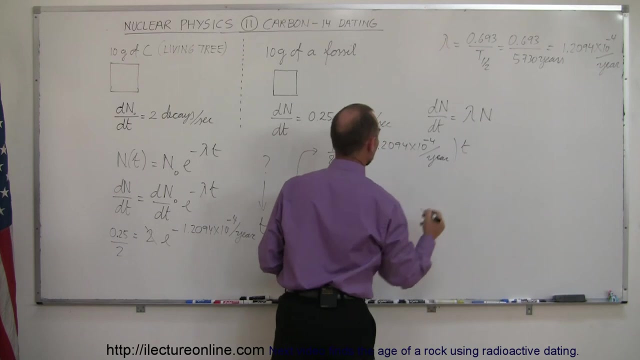 times. so, coming over here, I can say that 1.8 is equal to e, to the minus 1.2094 times 10, to the minus 4 per year times t. Now, of course we're going to take the natural log. 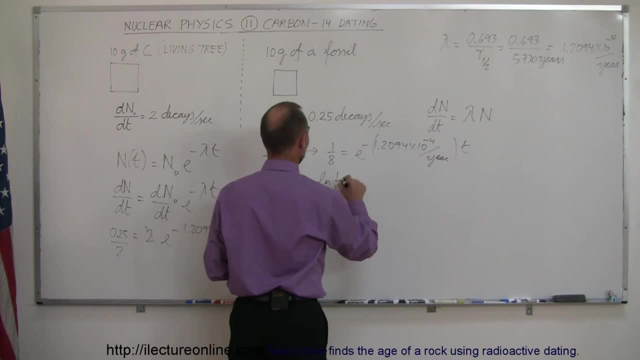 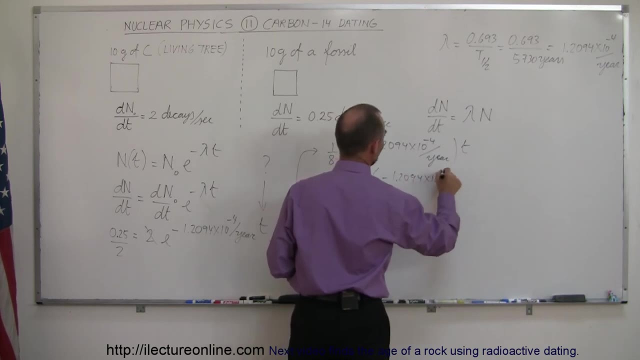 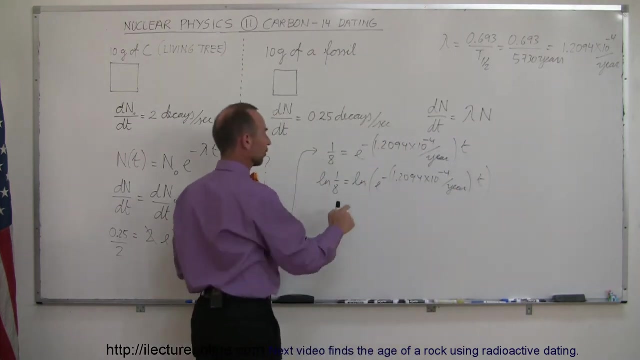 of both sides. so the natural log of 1.8 is equal to the natural log of e, to the minus 1.2094 times 10, to the minus 4 per year times t, like so, And of course this will negate. 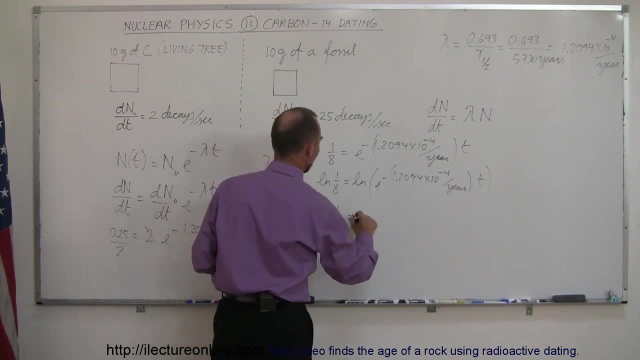 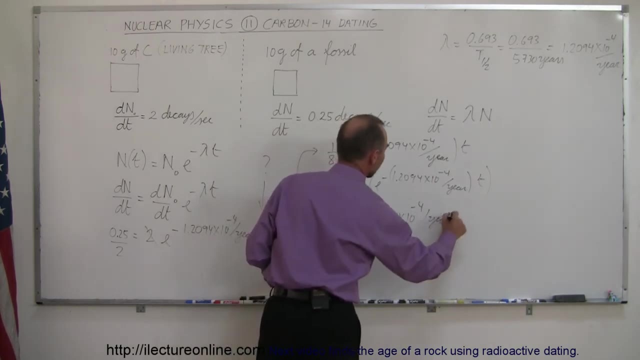 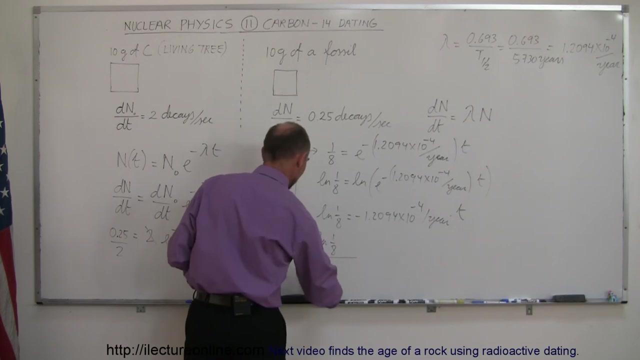 that. so we have the natural log of 1.8.. Is equal to minus 1.2094 times 10, to the minus 4 per year times t And, of course, dividing both sides by this quantity, right here we have the natural log of 1.8 divided by minus. 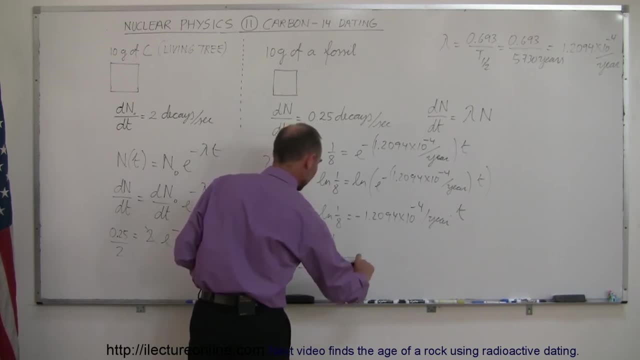 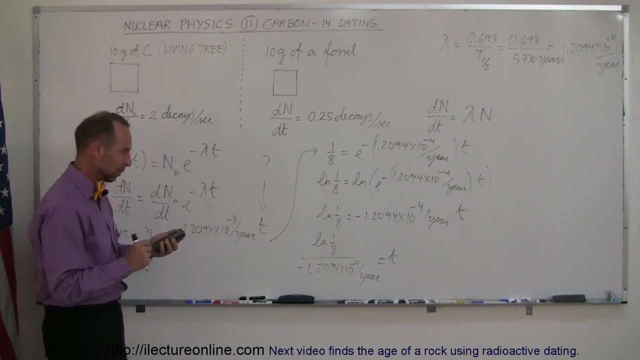 1.2094 times 10 to the minus 4 per year is equal to t, And all we have to do now is grab our calculator, plug those numbers in there, see what we get. So take the inverse of that, since I already have that in my calculator. 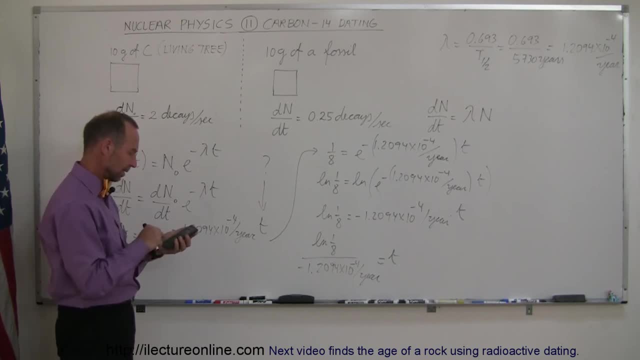 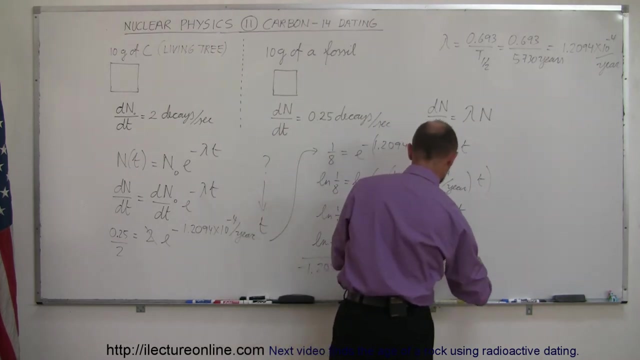 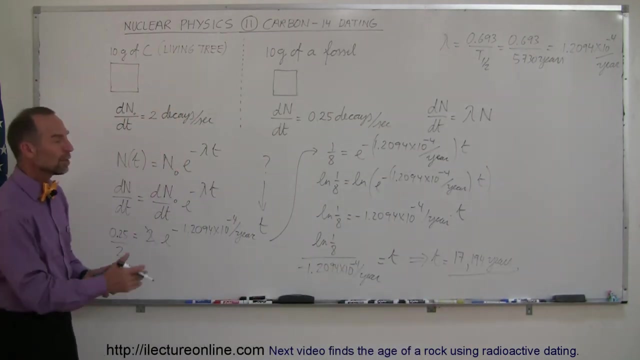 And multiply that times hmm, 1 divided by 8. And that is take the natural log of that And that's equal, And the answer I get is that the time elapsed, or the age of that fossil is equal to 17,194 years. Of course. how accurate is that method? Do we know it? 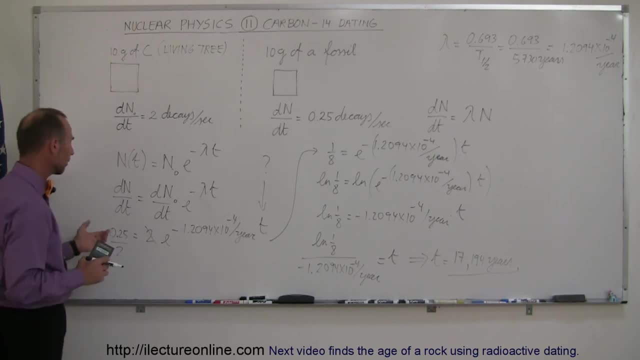 down to the nearest year? Of course not, because that all depends upon how accurately we're to measure the decay rates of the elements, and one of the big things about trying to measure the decay rate of a sample from a fossil is that there's natural radiation occurring around us all.